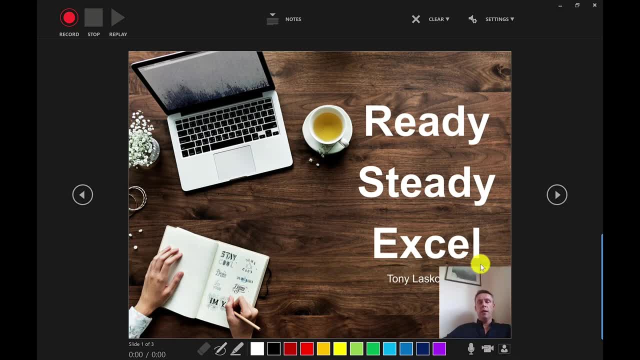 window will collapse. anyway, Let's keep it on. Don't worry about the position at this stage. you can always move it later. And you've got this mic button as well. so if you want to mute the mic or not, You've got a series of colors. I will come to that when we start the presentation. 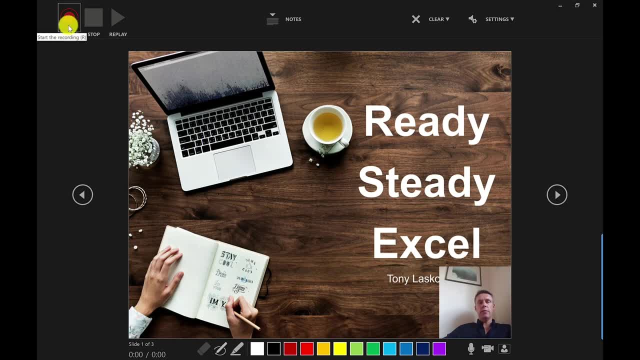 So that's everything. So I'm good to start recording. So up here I just press record. That's the countdown. So that's now recording. So it's going to be picking up my slide movement, my talking, the audio. So if I click next so I can be talking through this slide, You'll also notice up here in. 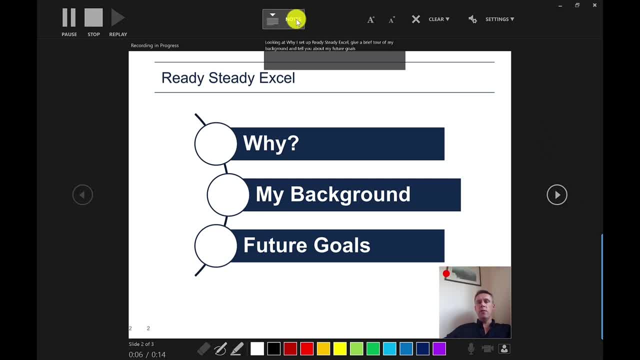 the middle. you've got your notes, So you can add notes to the slides and you can read it from here And this won't appear in the recording. You do have options here to make those notes bigger, depending on your eyesight. 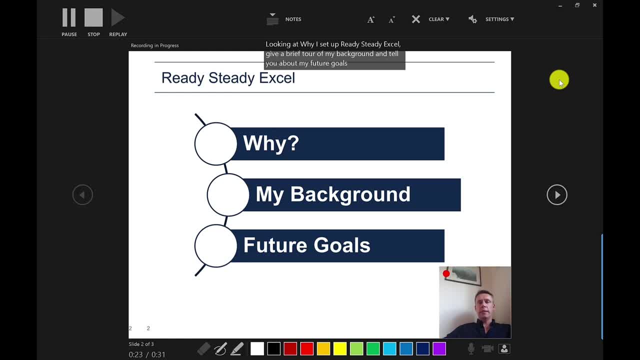 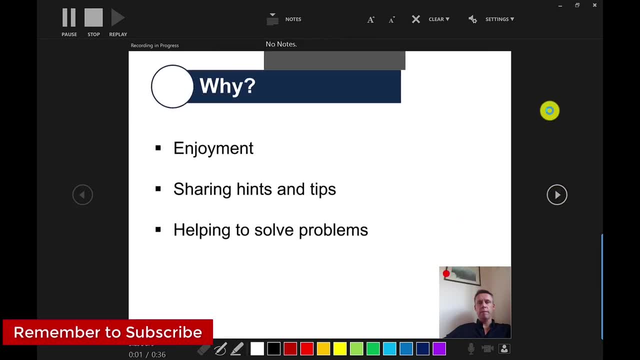 So here I am in my slideshow talking about this slide. So this is what I'm going to be covering today, And then, if I click next over here, I can say why. why I set up Ready, Steady Excel, And down here at the bottom you've got these. 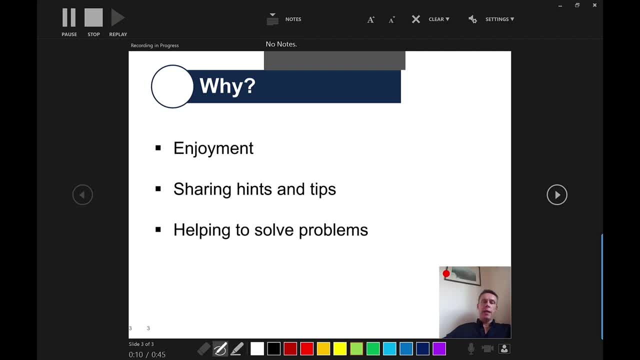 colors. So if you needed to, you can use these colors and then you can need it just right on the slides themselves And this will appear on the recording. Okay, So once you've done with the recording up here at the top, you've got the option to stop it. 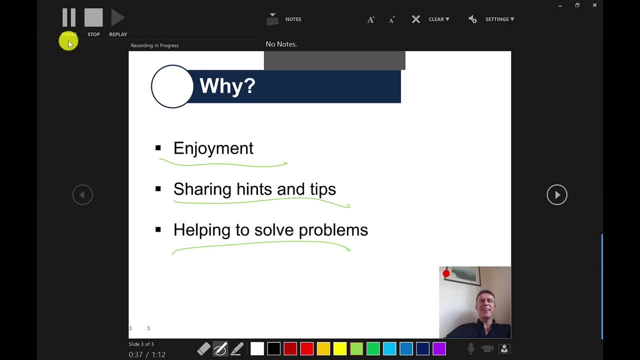 You also have the option to stop the recording. So you've got the option to stop the recording. You've got the option to stop the recording, And then you've got the option to stop the recording. You've got the option to pause. So maybe if the doorbell rings and you need to answer the door, 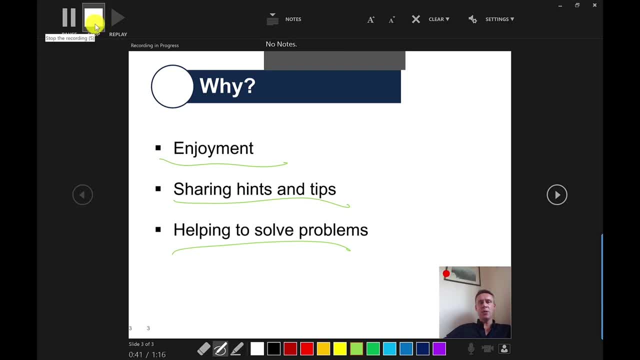 you could pause it and then return, But I'm happy with this, So I'm just going to press stop. You've got the option to replay it, So if you just want to check how it went, you can do that. But I'm confident I'm going to take a chance, And so I'm just going to X out of this one. 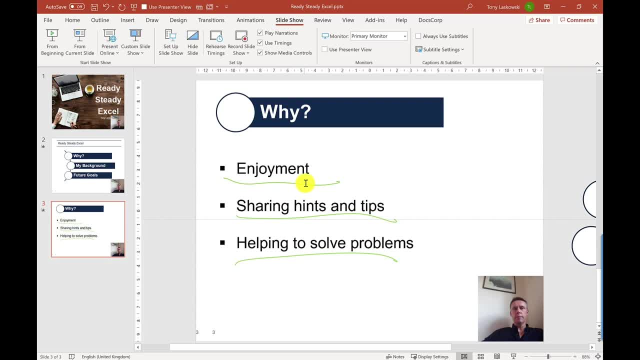 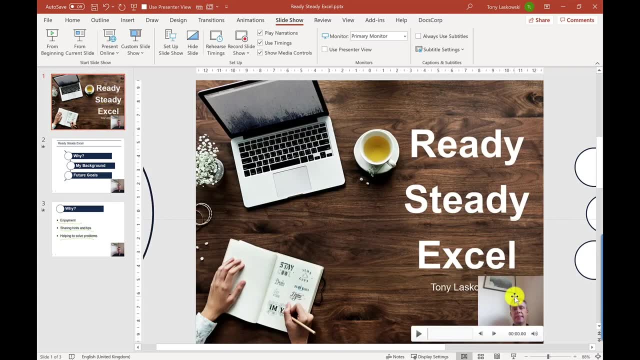 As you can see, it's brought across the annotation there. If you did change your mind, you wanted to delete these. you can just click on them to delete them off. You'll also notice that on each slide you've got the video, So maybe I don't want to delete them.